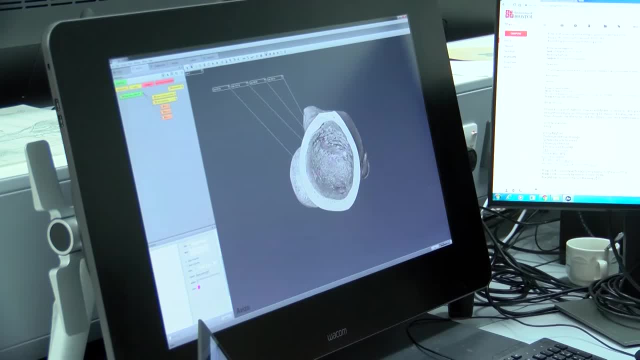 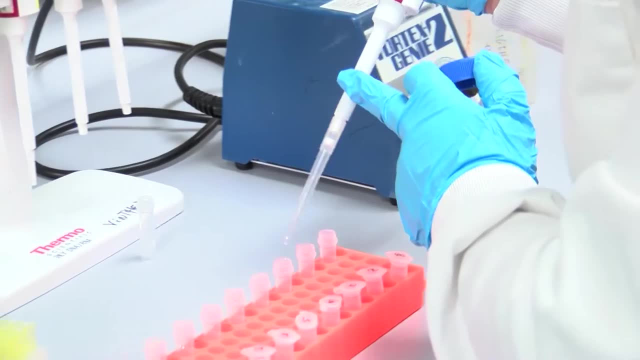 have a tomography lab with ten high-end workstations with software installed that will enable you to do image analysis and biomechanical analysis. We have wet lab facilities for molecular paleobiology. We also have all the computational expertise that you would need to do things like macroevolution. 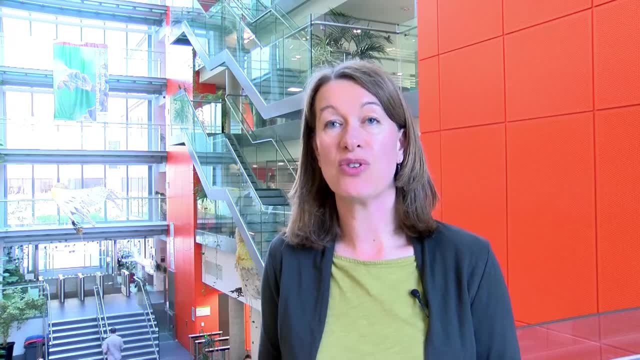 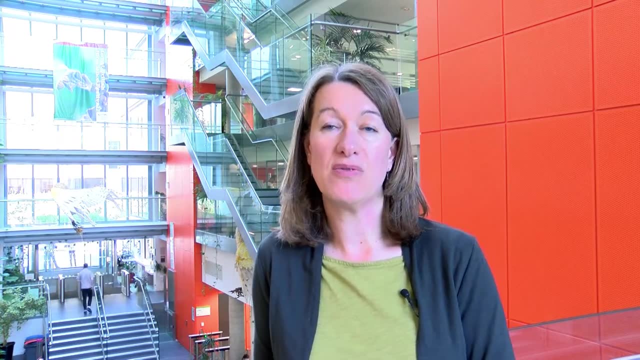 phylogenetics and phylogenomics. Our students join us from a wide range of different backgrounds. We have biologists, geologists, chemists, physicists, biologists, biologists, biologists, biologists- and we'll provide you with a range of taught units that will all bring. 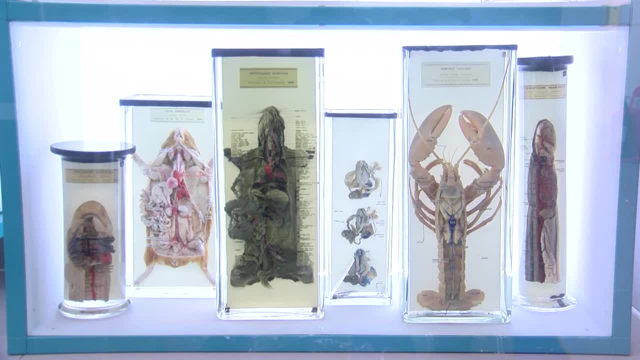 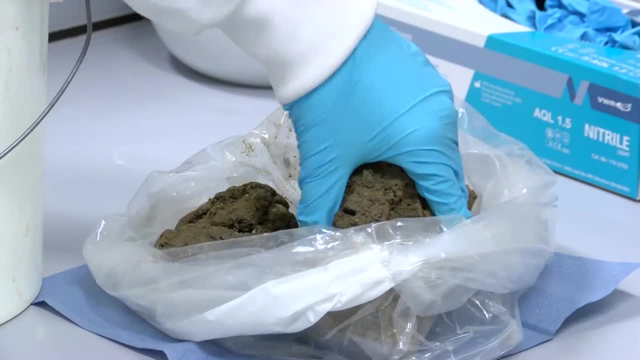 you up to the same level. So, for example, if you come from a geology background, we'll provide you with an option in evolutionary biology. Likewise, if you come from a biology background, we'll provide you with a taught course in geology that will bring you up to the level. 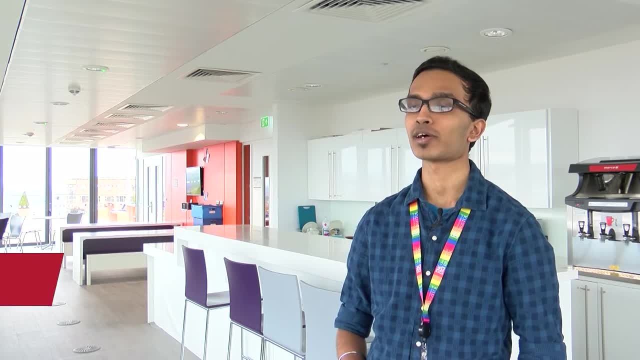 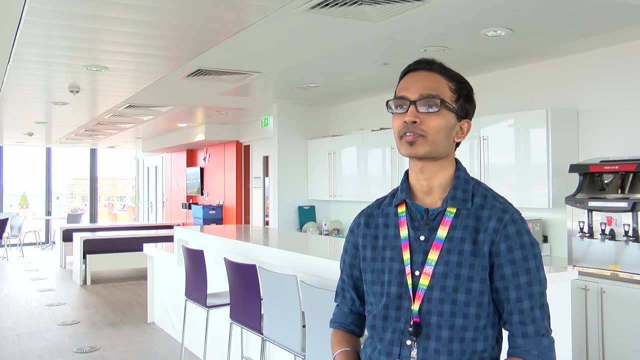 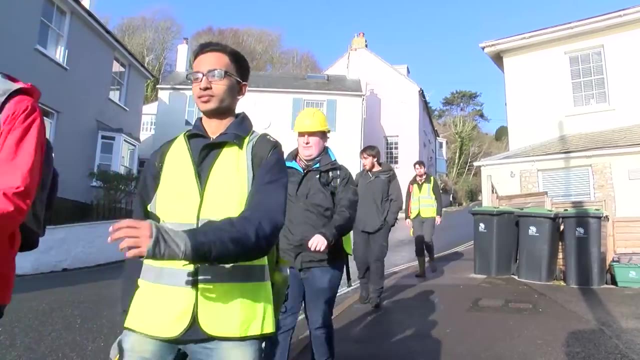 of a research paleobiologist. I'm one of the current paleobiology master's students. I'm currently working on the skull biomechanics of Mesozoic terrestrial crocodilians with Professor Emily Rayfield. Going to Bangalore or anywhere in the world is a big move. You're coming to a new city. 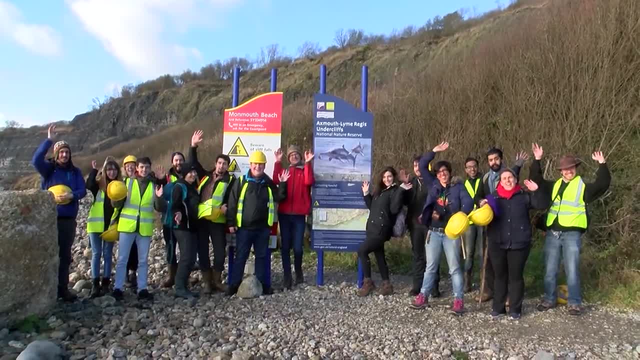 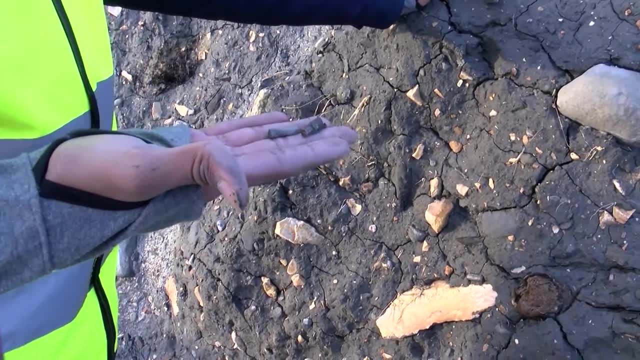 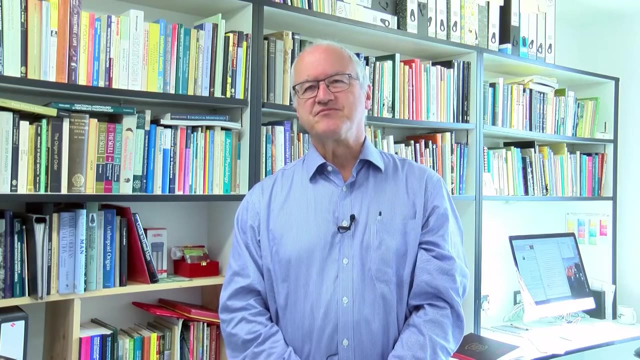 and a new country. The MSc here in Bristol is the largest of its kind, so you quickly make lots of friends. We're all from different places and have different backgrounds, but we share the same passion for fossils, so you feel right at home Over the years. we're really pleased that so many of our students have been successful. 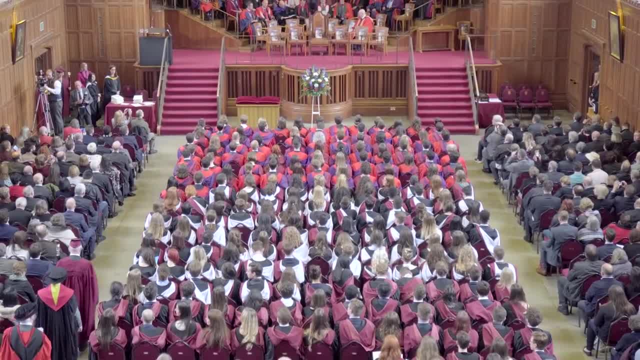 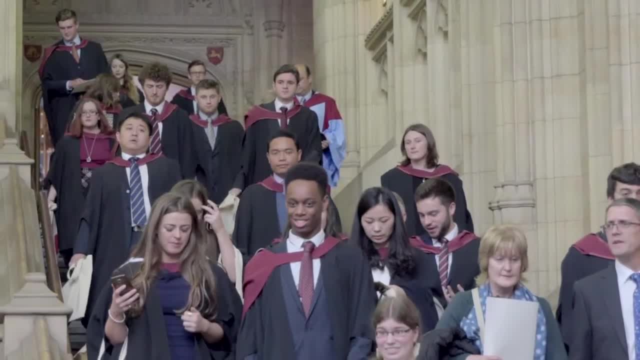 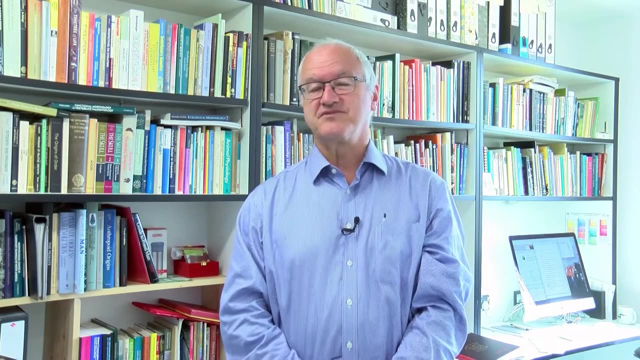 At least a third have gone on to do PhDs, and a lot of the training we offer, of course, is directed towards that. We're pleased to keep as many students here to do PhDs in Bristol as we can, But equally a large number go to work in museums and education and other areas of commerce. 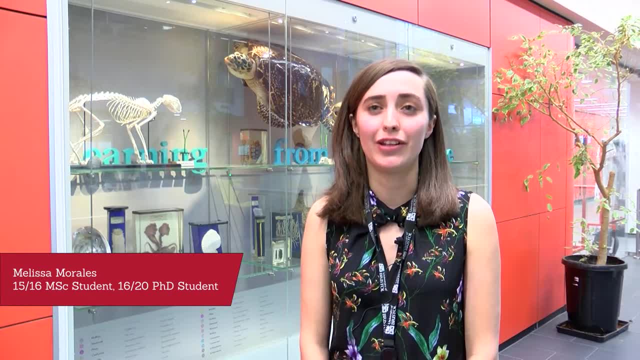 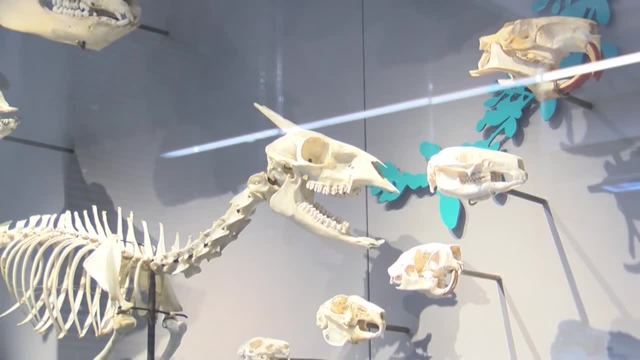 My name is Melissa and I am currently doing my PhD here at the University of Bristol. Two years ago I did my master's degree and I was working on ungulate community dynamics under the supervision of Professor Christine Janis. Upon completion of my project, I presented 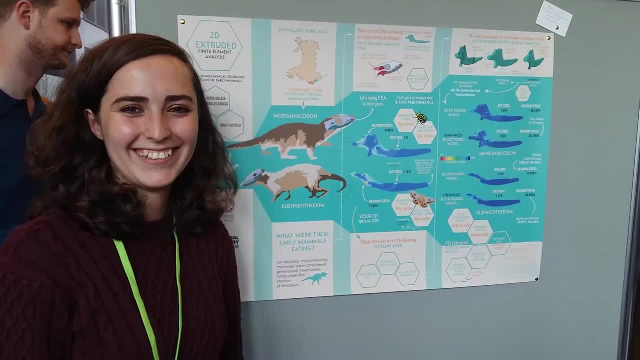 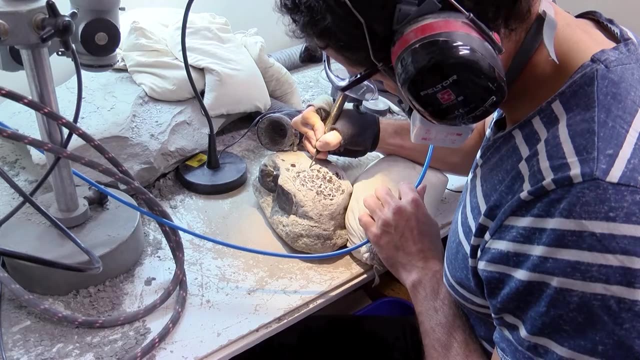 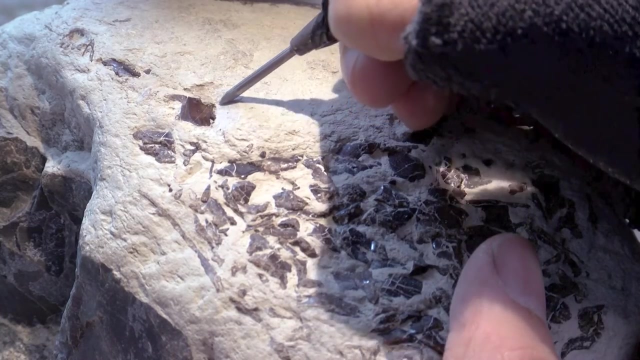 my results at an international paleontological conference. A great strength of the degree is that we focus a lot on methods. We teach you all of the computational and laboratory methods that you would need to be a successful paleontologist, But many of these methods are of great use in a much wider range of employment.